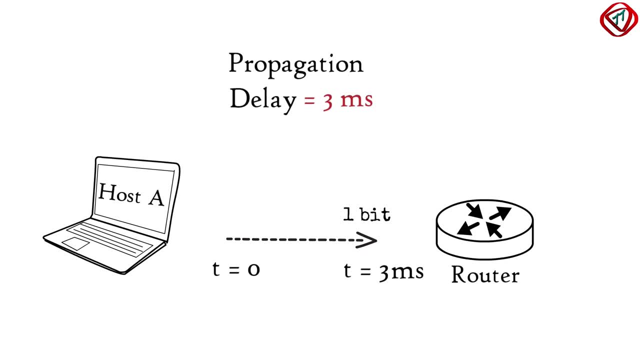 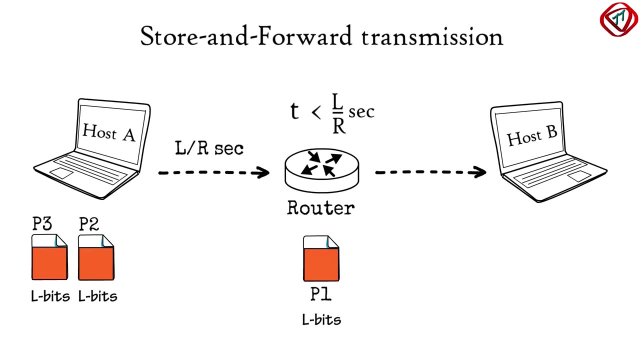 router is 3 ms, It is called propagation delay. If the propagation delay is 0, then the first bit is available to the router at the same time host A transmits it. In the current case the host A completes sending the first packet at time L by R seconds. So if the propagation 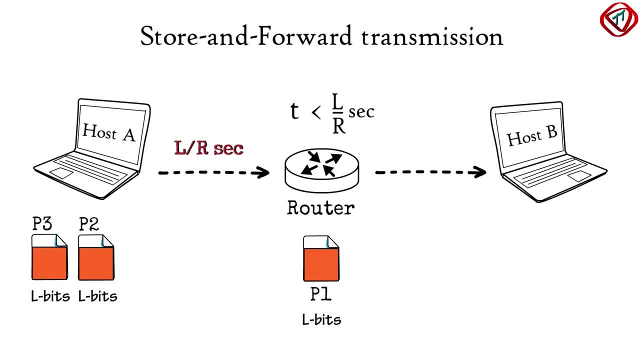 delay is 0,. the router receives stores and starts sending the packet P1 to the host B at the same time L by R seconds. Now the router is also transmitting at a rate of R bits per second, Since there are L bits in one packet. so host B receives the packet. 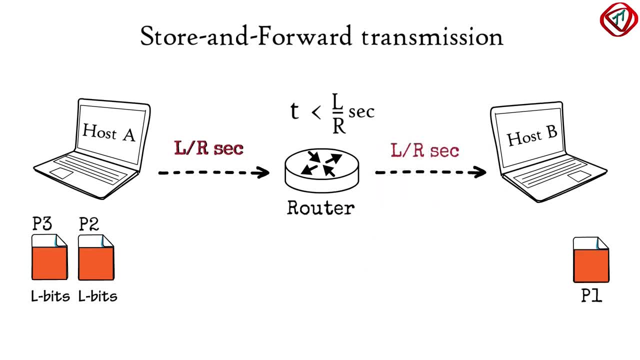 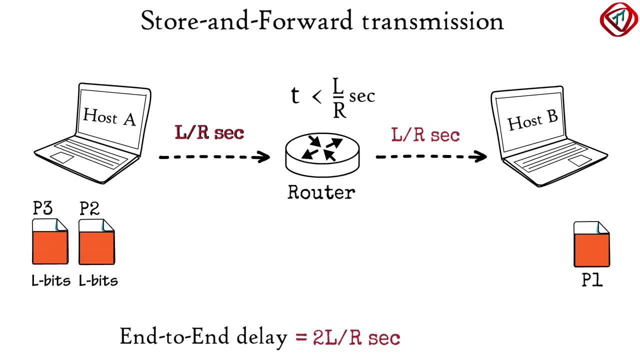 P1 after sending the first packet at time. L by R seconds. After additional L by R seconds. Hence the total end-to-end delay in receiving the first packet is 2 L by R seconds. In general it is N L by R seconds, where N is the number. 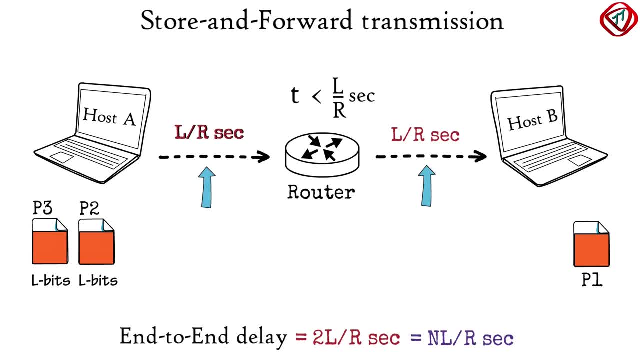 of links. In our case, host A has 3 packets At time, L by R seconds. the router has received the packet P1 and has started sending it to the host B At the same time. host A transmits the packet P1 to the host B At the same time. host A. 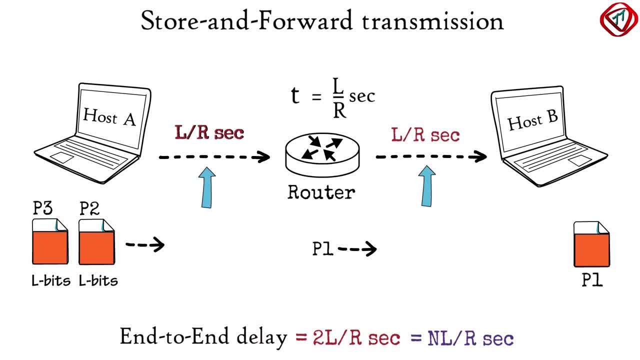 transmits the packet P1 to the host B At the same time. host A transmits the packet P1 to the host B At the last time, L by R seconds. host A has started sending the packet P2 to the router. 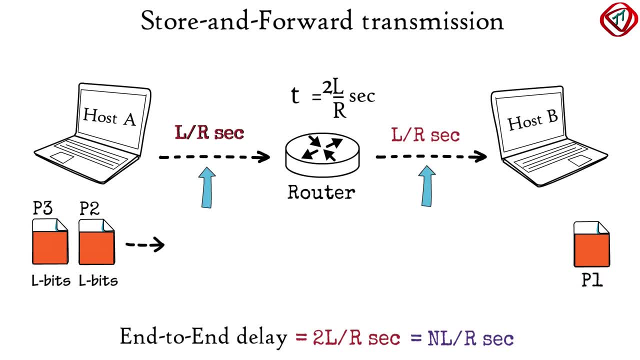 So at time, 2 L by Rs, host B receives the first packet, P1, and the router receives the second packet, P2. At 3 L by R seconds, host B receives the second packet and the router receives the third packet. At last, 4 L by R seconds, the host B receives the third packet. 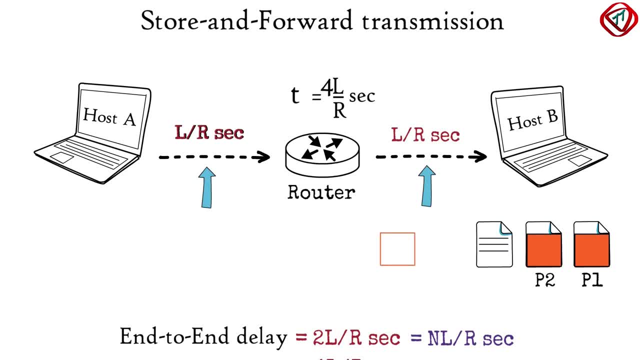 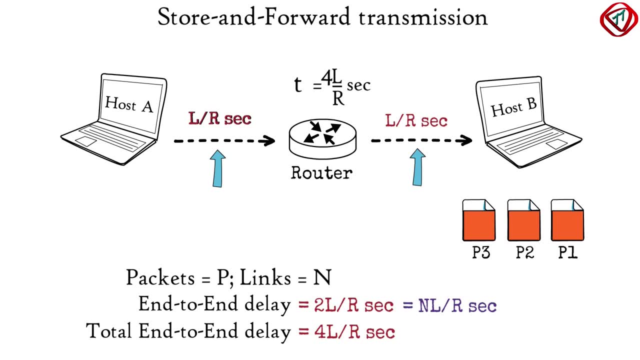 In general, if there are six past- Natalya Productions packages, all of them are echelons by 7, Nor label highest Ad granny. If there are P packets and N links, the total end-to-end delay is N plus P minus 1 into L by R seconds. 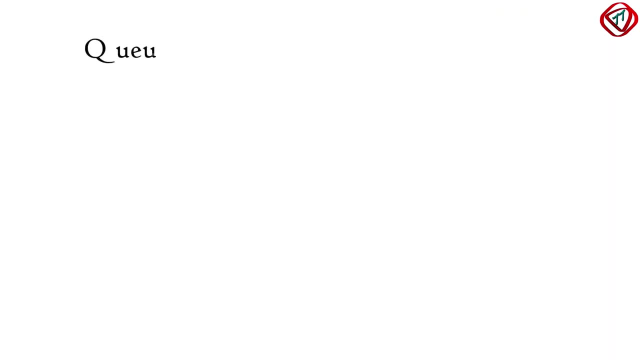 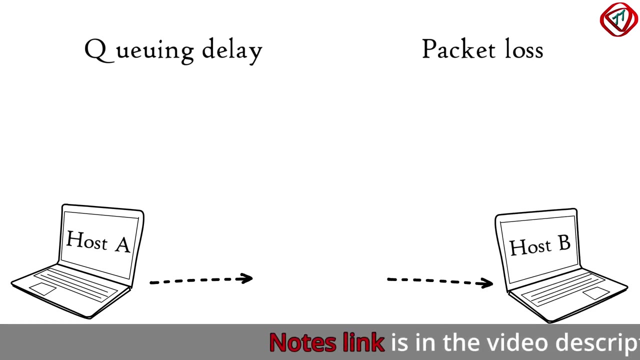 Along with this store and forward. delay, queuing delay and packet loss may occur. Suppose the host A is sending a file to host B via a packet switch. The router is sending data to host B at a transmission rate of 10 Mbps. 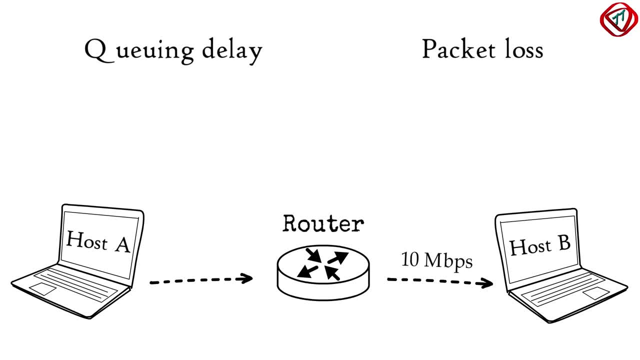 Till the host A's transmission rate is less than or equal to 10 Mbps. no queuing will occur. In case host A's transmission rate exceeds 10 Mbps, for a moment the incoming packets have to wait in the buffer present in the router and forms a queue. 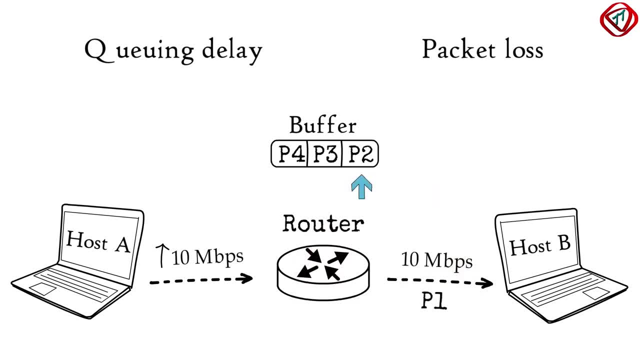 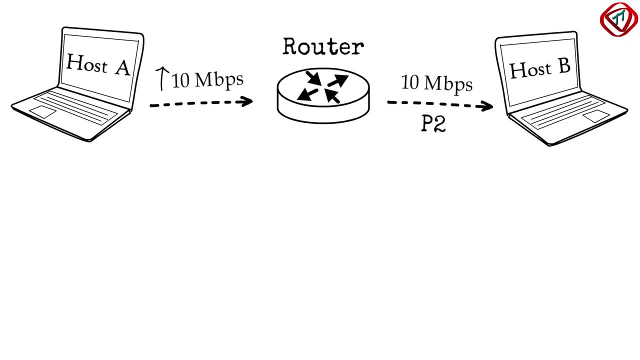 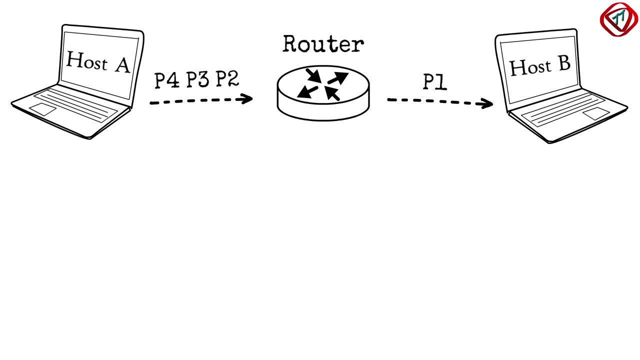 The time till when the incoming packet waits in the queue before transmission is called queuing delay. Queuing delay can also occur. Queuing delay can also occur in cases where host A is sending packets to the router but the router is busy in sending packets received from host C. 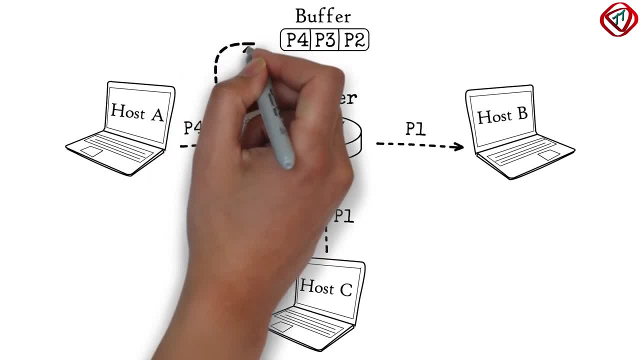 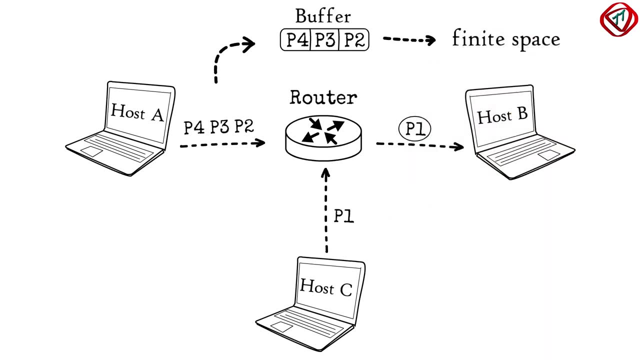 The packets received from host A will queue in the buffer till the previous transmission is over. Since the buffer has a finite space, cases may occur where the incoming packet may find the buffer completely filled. Either the incoming packet or the one present in the buffer is dropped off. 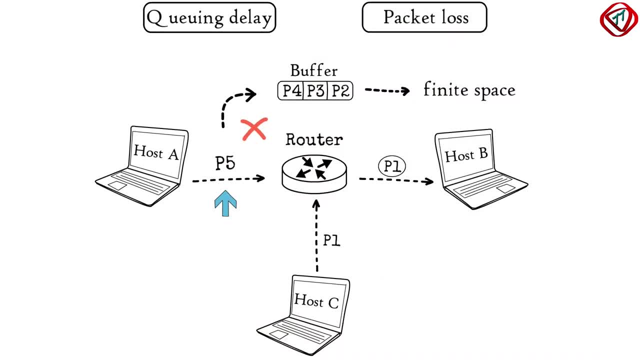 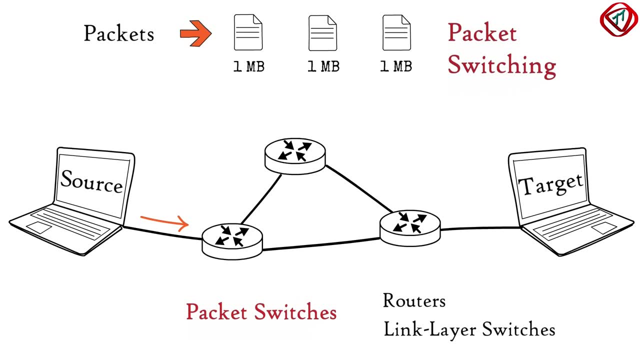 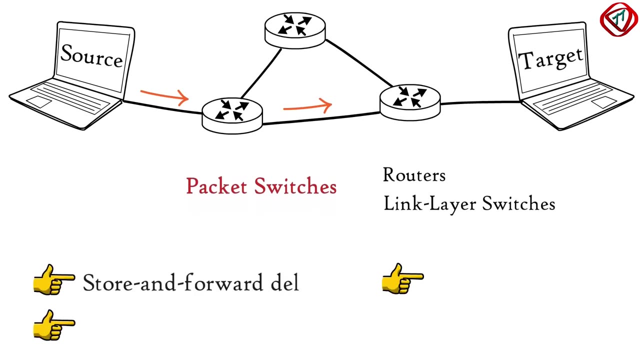 It is called packet loss. Till now we have learnt that in packet switching, packet switches receive packets at one communication link and forwards it to another communication link. During this process it may suffer store and forward delay, queuing delay or packet loss. 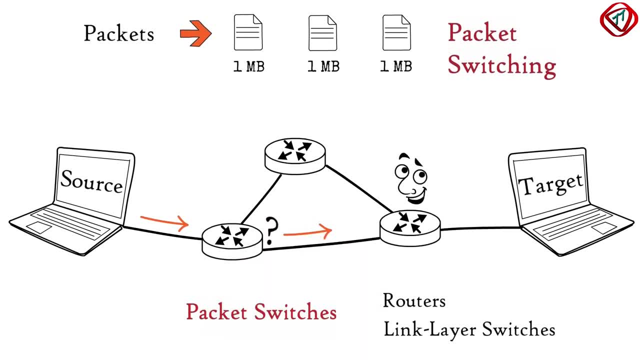 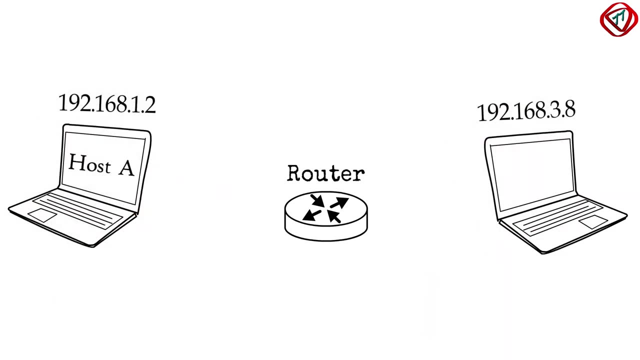 But how packet switches know to which communication link the incoming packet should be forwarded. Here forwarding tables come into picture On the internet. every device has a unique address, known as IP address, When host A sends a packet to host B. 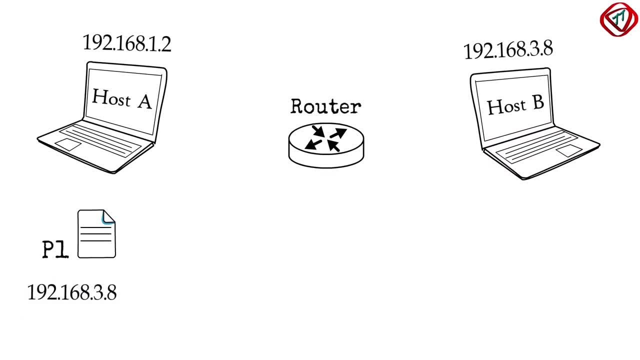 it maintains the IP address of host B in the packet's header. Every router has a forwarding table. It maps the portion of IP address or network address to the router's link interface. When a router receives a packet, it matches the prefix of the packet's destination address.